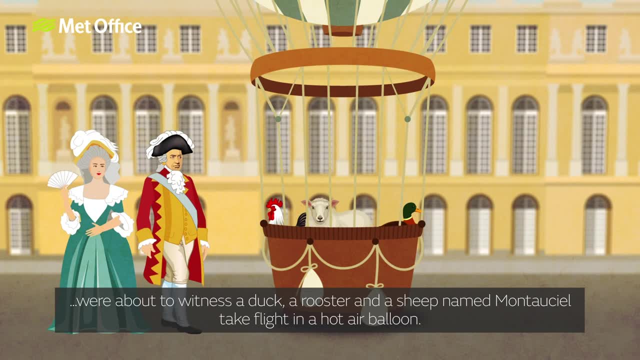 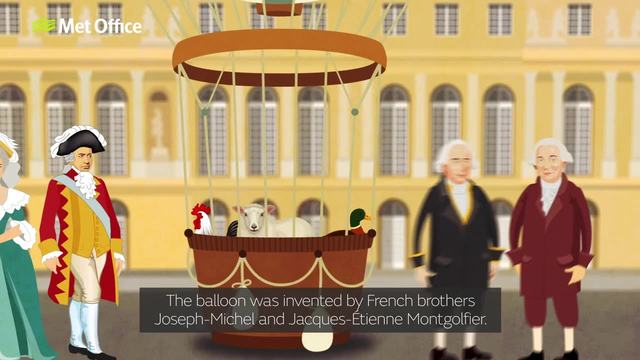 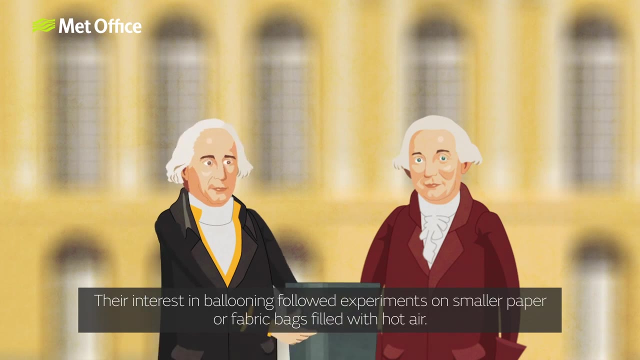 sheep named Montaussiel take flight in a hot-air balloon. The balloon was invented by French brothers, Joseph Michel and Jacques-Étienne Montgolfier. Their interest in ballooning followed experiments on smaller paper or fabric bags filled with hot air. Having successfully launched an unmanned hot-air, 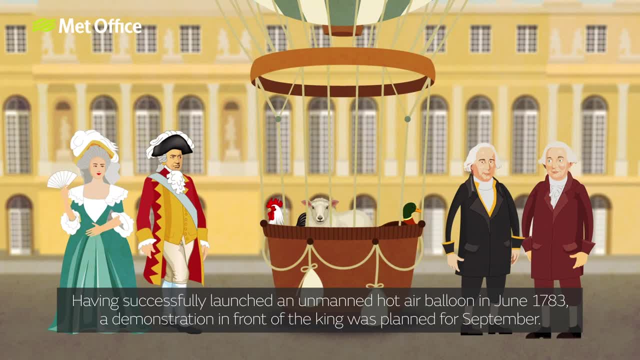 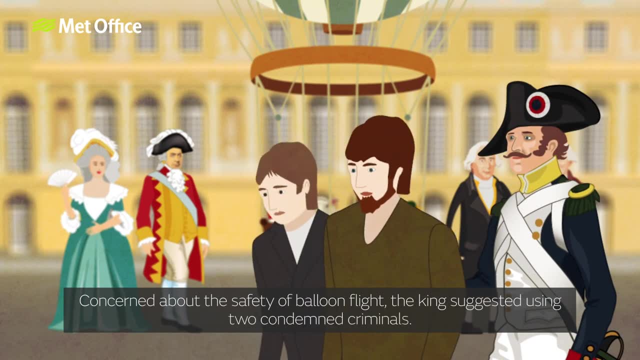 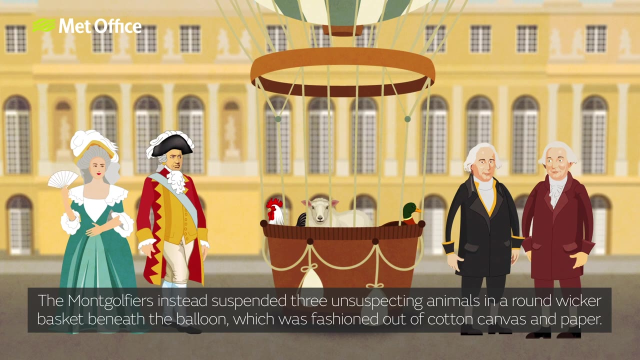 balloon in June 1783. a demonstration in front of the King was planned for September. Concerned about the safety of balloon flight, the King suggested using two condemned criminals, The Montgolfiers in. instead suspended three unsuspecting animals in a round wicker basket beneath the balloon. 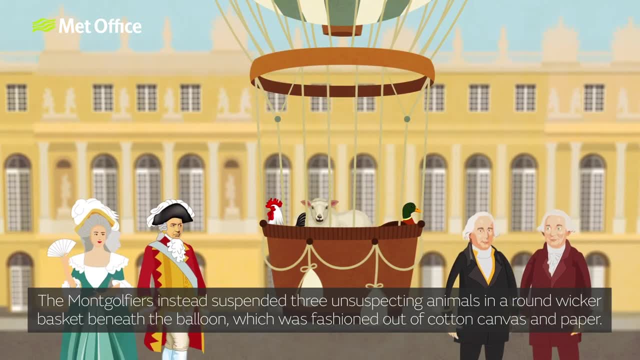 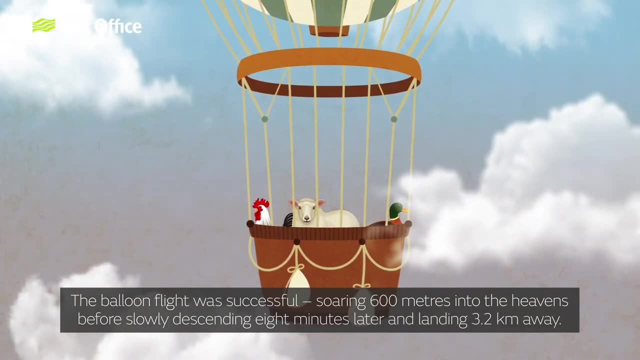 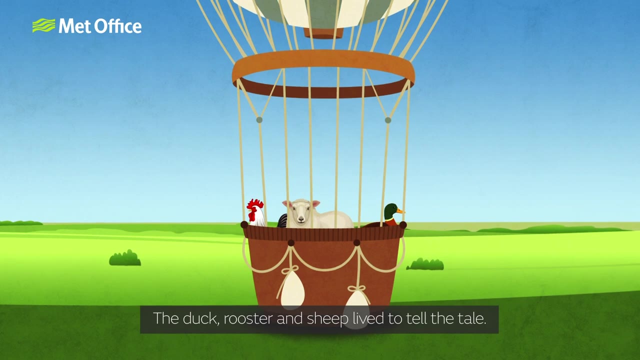 which was fashioned out of cotton, canvas and paper. The balloon flight was successful, soaring 600 metres into the heavens before slowly descending eight minutes later and landing 3.2 kilometres away. The duck rooster and sheep lived. to tell the tale, They were. 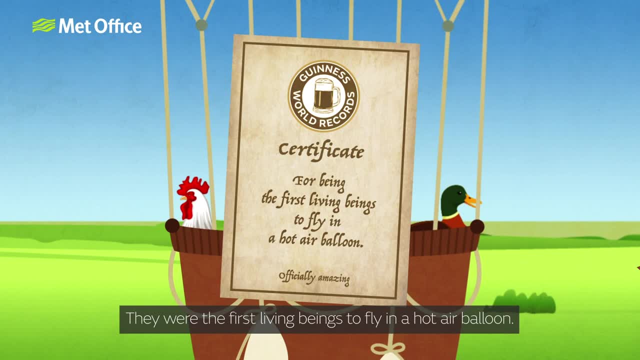 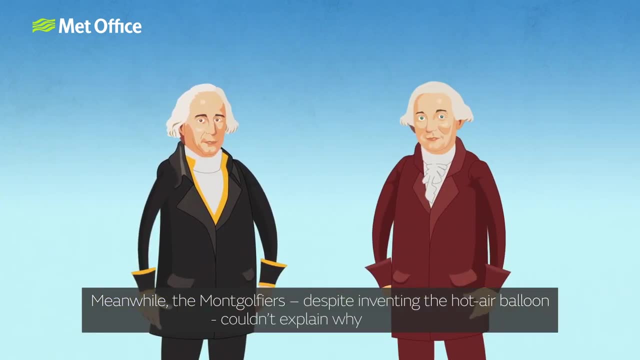 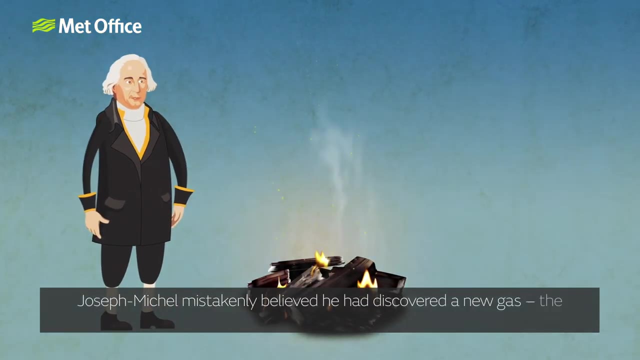 the first living beings to fly in a hot-air balloon. Seven flights were completed later that year. Meanwhile, the Montgolfiers, despite inventing the hot-air balloon, couldn't explain why it floated. Joseph Michel mistakenly believed he had discovered a new gas, the Montgolfier gas, which was lighter than air and released. 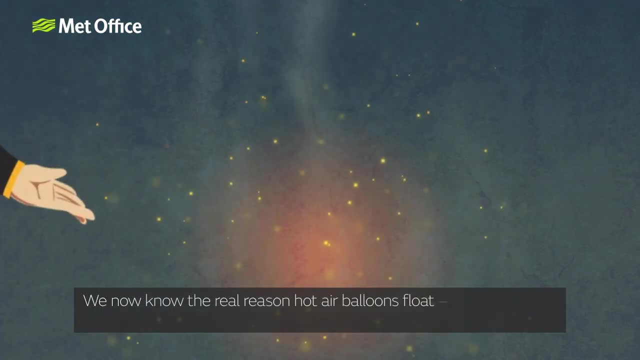 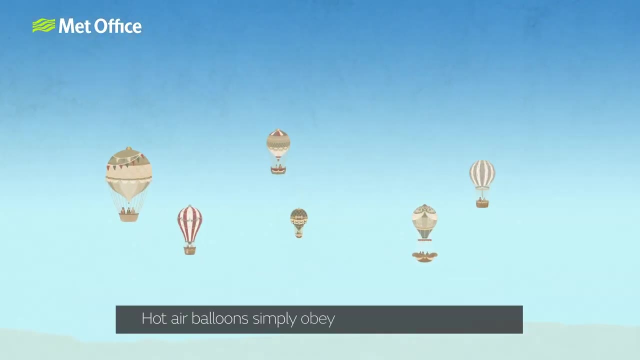 from burning embers. We now know the real reason: hot-air balloons float and it's nothing to do with an imaginary gas. Hot-air balloons simply obey certain rules and rules of the natural world, and their own requires of them. They themselves have a specific purpose and they are the life of 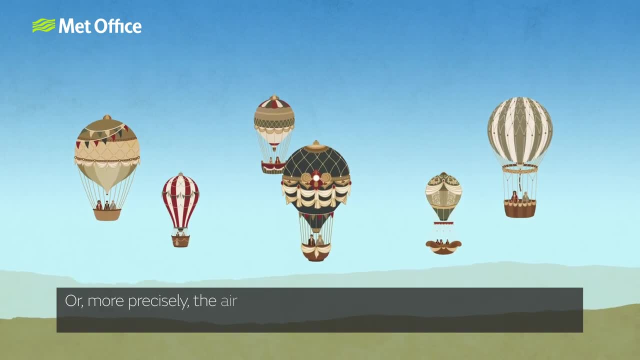 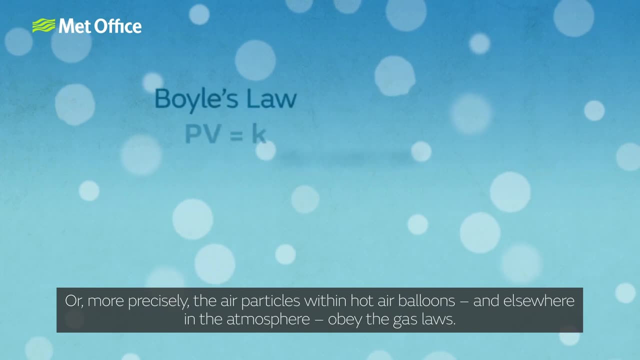 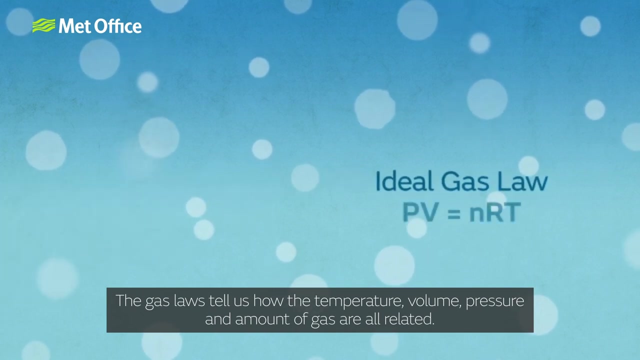 the human being. They are the life of the human being for which they come from, When they laws of physics, or more precisely the air particles within hot air balloons and elsewhere in the atmosphere, obey the gas laws. the gas laws tell us how the temperature, volume, pressure and amount of gas are all related. the gas laws were 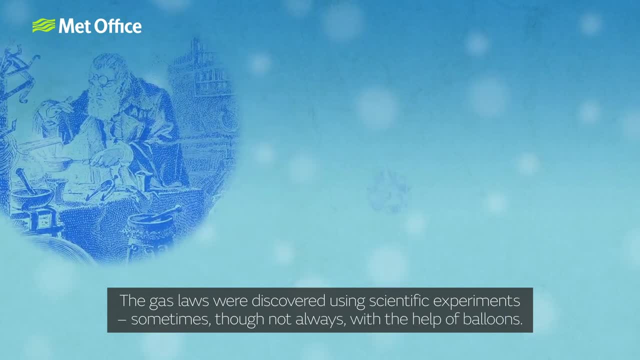 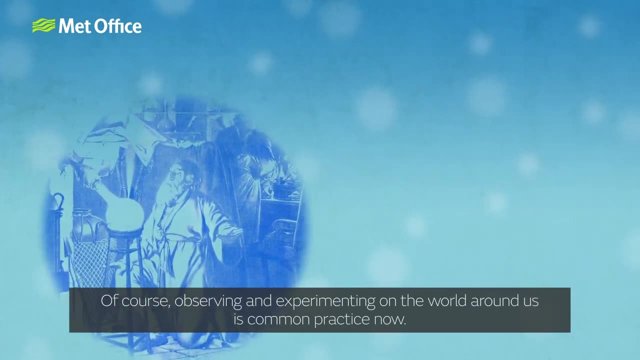 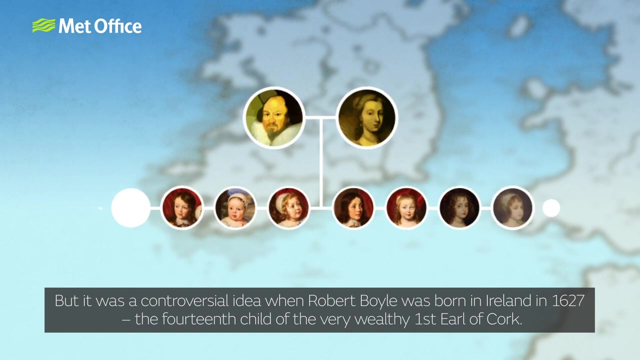 discovered using scientific experiments, sometimes, though not always, with the help of balloons. of course, observing and experimenting on the world around us is common practice now, but it was a controversial idea when Robert Boyle was born in Ireland in 1627, the 14th child of the very wealthy first Earl of 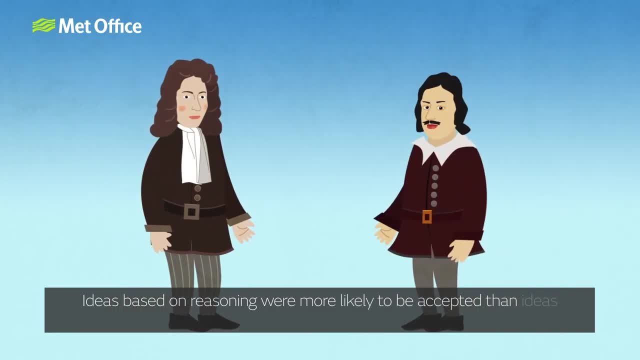 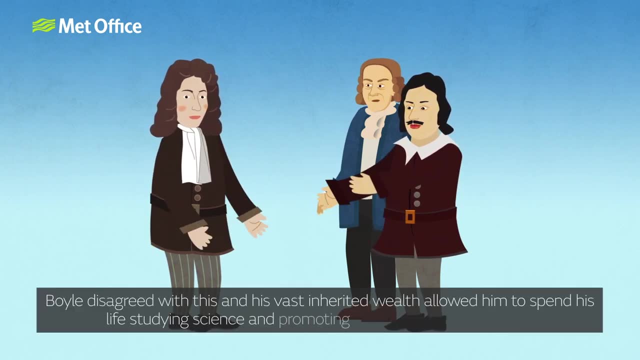 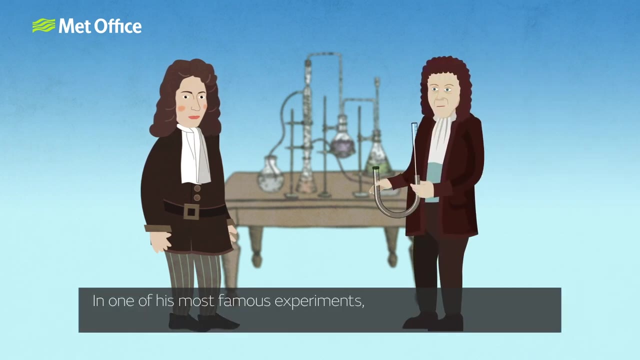 Cork, ideas based on reasoning were more likely to be accepted than ideas tested in experiments. Boyle disagreed with this, and his vast inherited wealth allowed him to spend his life studying science and promoting the experimental method. in one of his most famous experiments, a j-shaped tube was built by his assistant, Robert hook, with mercury. 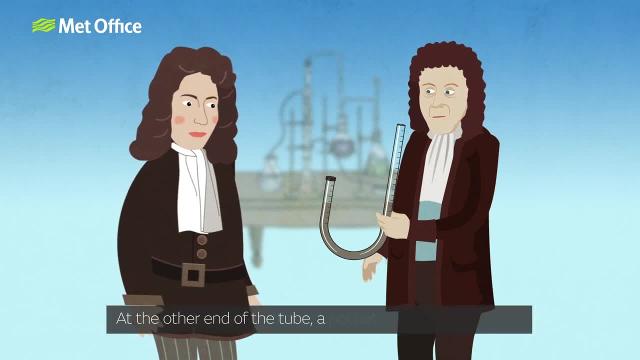 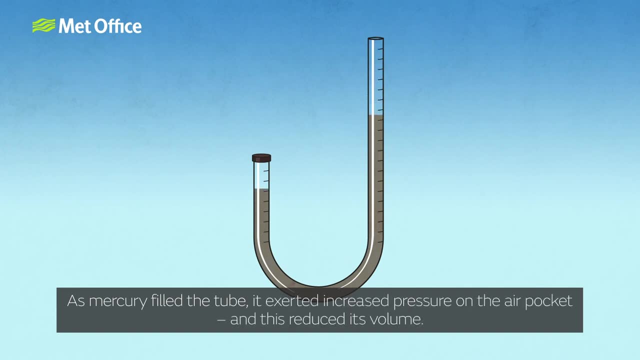 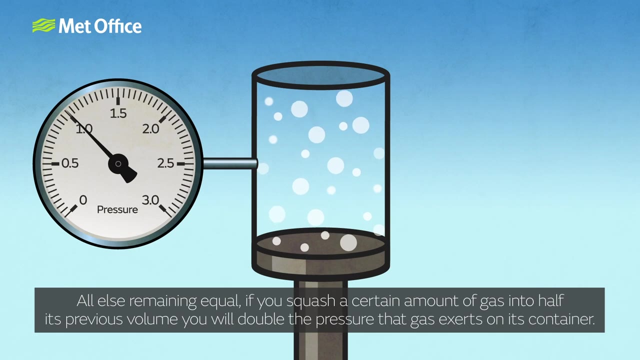 poured into one end. at the other end of the tube, a pocket of air was contained. as mercury filled the tube, it exerted increased pressure on the air pocket and this reduced its volume, all else remaining equal. if you squash a certain amount of gas into half its previous volume, you will double the pressure that 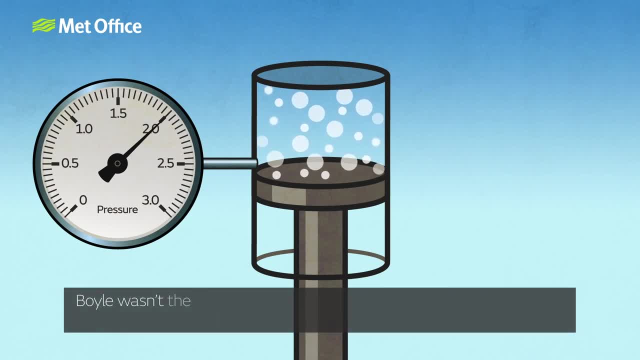 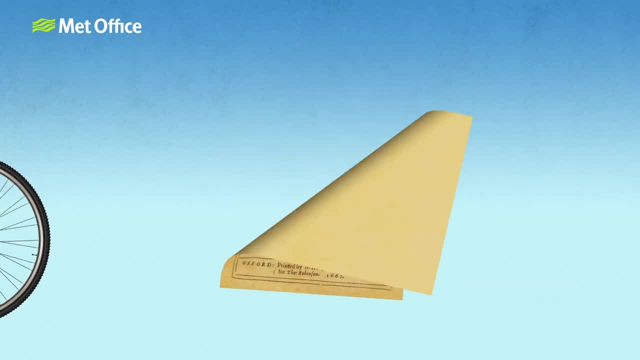 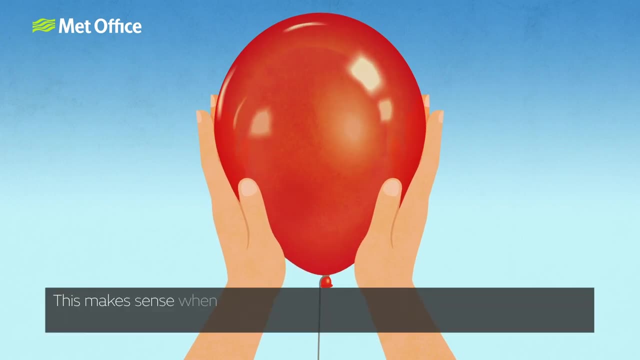 gas exerts on its container. Boyle wasn't the first to test these ideas, but he was the first to publish his findings, now known as Boyle's law. you can feel the effect of Boyle's law whenever you squeeze a bike tire or squash a balloon. this makes sense when we 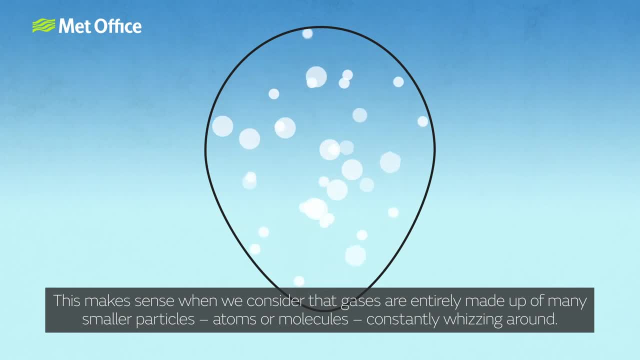 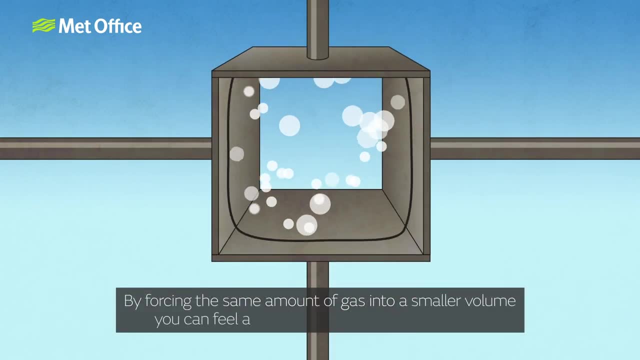 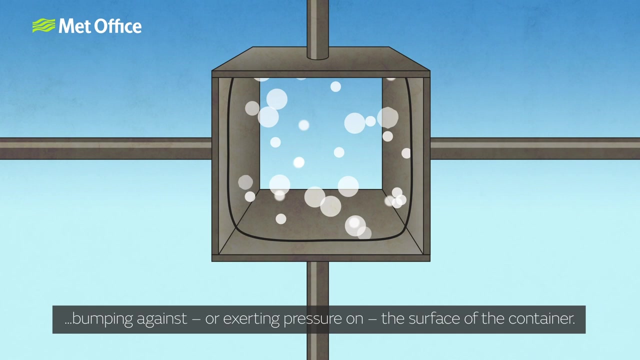 consider that gases are entirely made up of many smaller particles, atoms or molecules, constantly whizzing around. by forcing the same amount of gas into a smaller volume, you can feel a higher concentration of particles bumping against or exerting pressure on the surface of the container. how fast or 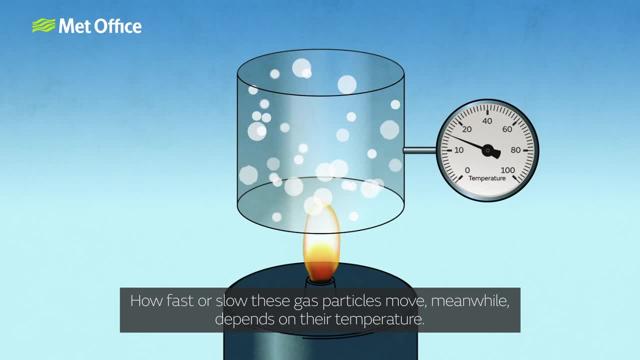 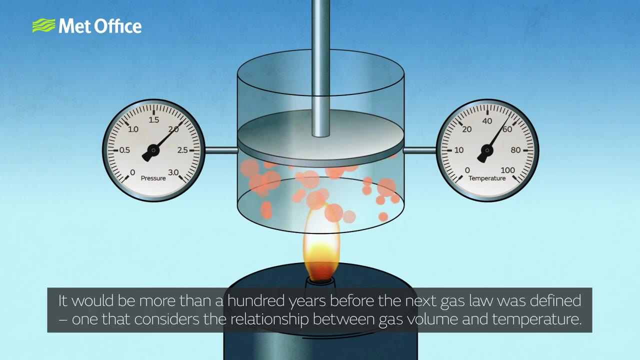 slow these particles move meanwhile depends on their temperature. in fact, that's essentially how temperature is defined. Boyle's law assumes that the amount of gas and the temperature of that gas are kept constant. it would be more than a hundred years before the next gas law was defined, one that 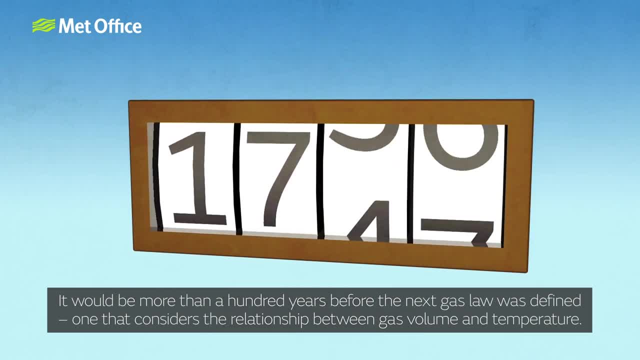 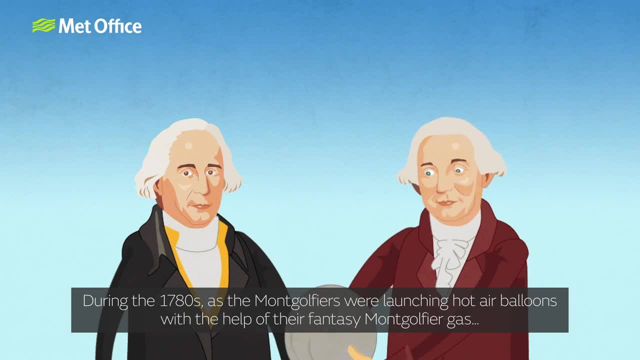 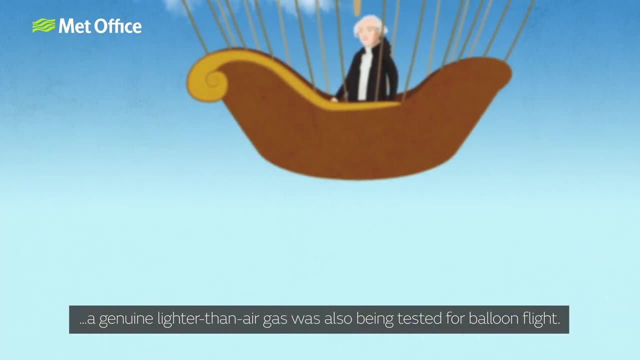 considers the relationship between gas volume and temperature. during the 1980s, as the Montgolfiers were launching hot air balloons with the help of their fantasy, Montgolfier gas, a genuine, lighter than air gas, was also being tested for balloon flight. on the 1st of December 1783, ten days after the first manned hot 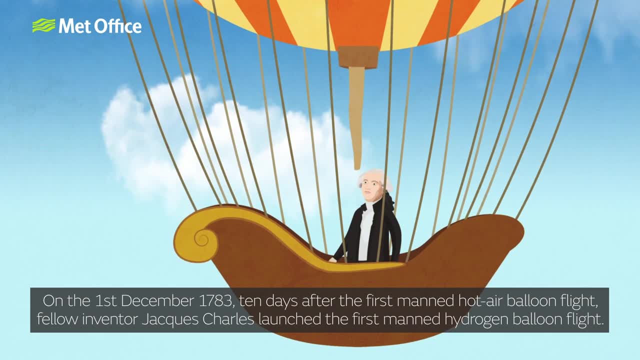 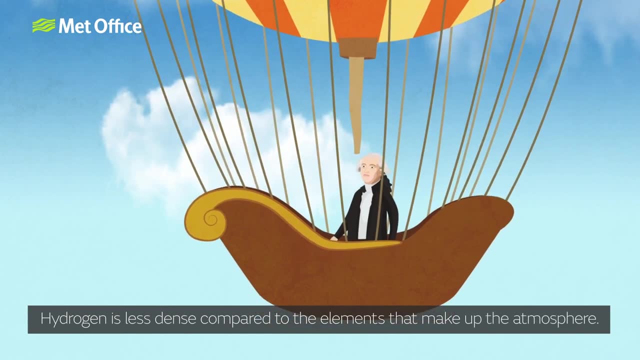 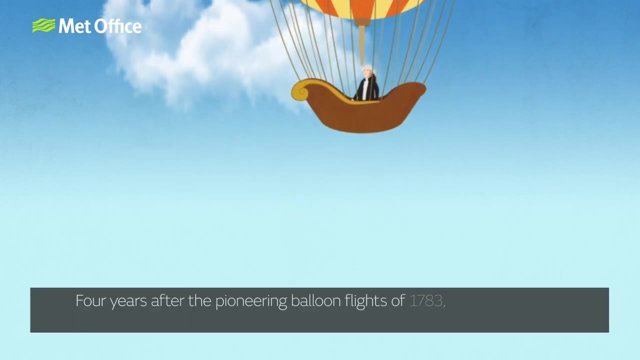 air balloon flight fellow inventor, Jacques Charles launched the first manned hydrogen balloon flight. hydrogen is less dense compared to the elements that make up the atmosphere, but what if it were also heated? would it become even lighter? four years after the pioneering balloon flights of 1783, Charles